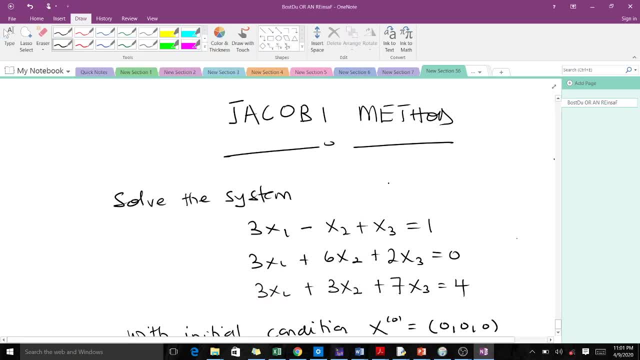 Welcome to today's lecture. So on today's lesson we are going to learn the Jacobi method. So remember, the Jacobi method is an iterative method for solving systems of linear equation. We are going to illustrate the Jacobi method using this example here. 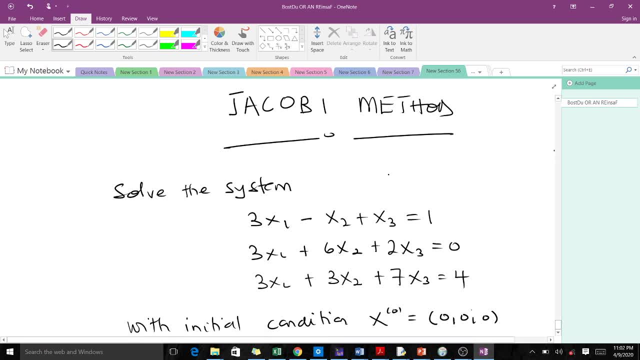 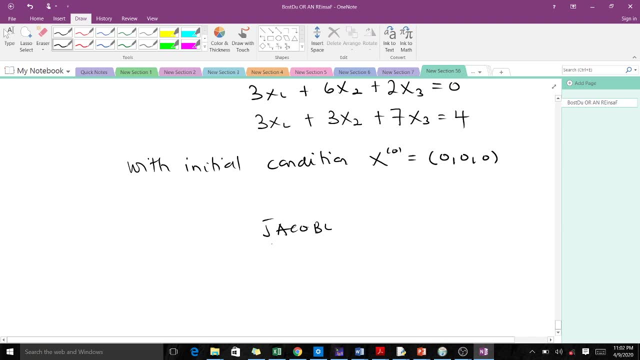 So we say: we solve this system with this particular initial condition, So with the Jacobi method. if you want to use the Jacobi method to solve it, these are the steps we follow. So the first step is that we make S1 the subject in our first equation. 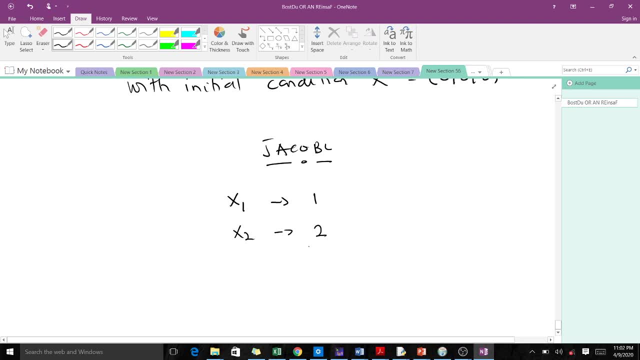 Then we make S2 the subject in our second equation, Then we make S3 the subject in the third equation. So after doing these manipulations, then the next thing we do is that we start with our iterations. So mostly we are being told to do just the iteration. 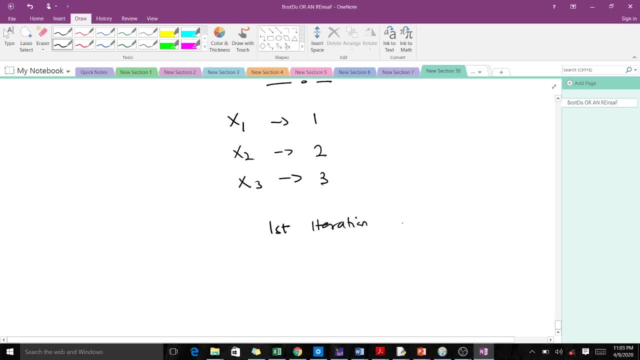 So for the first iteration, we will use our initial condition to get a new set of what X's, which will be X1. So after doing the first iteration, we are going to get S1. and new set of X's. 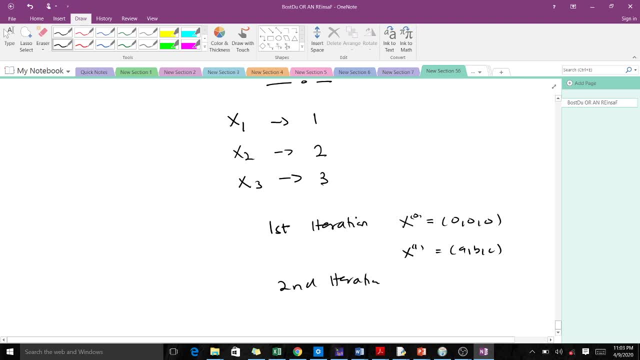 Then in the second iteration we will use these set of X's to get a new set of X's again. Then in the third iteration we will use the values for the second iteration to get our new set of values. So if we are being told to do 3 iterations, 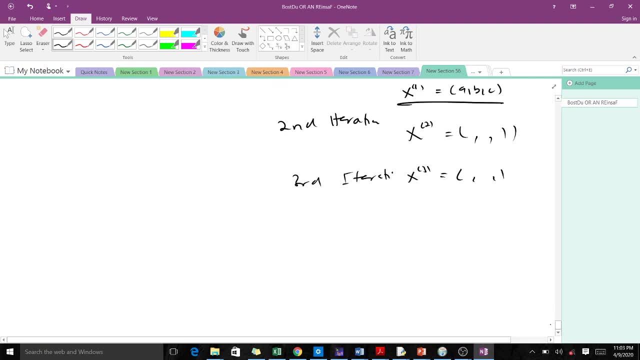 then that means our values in the third iteration will be detonged- will be the approximate solution to the system of linear equation given. so for the system that we have above, when we use the jacobi to solve it, the first thing we are supposed to do is to make s1. 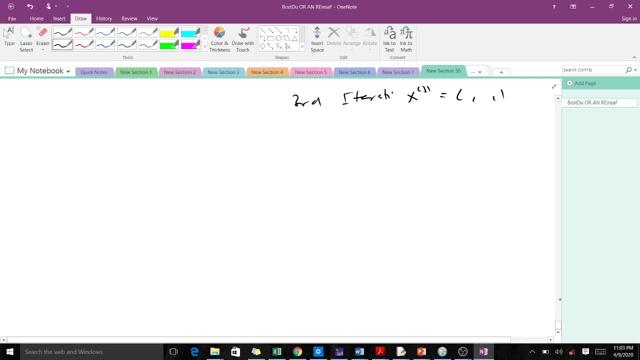 the subject in equation one, s2 in equation two and s3 in equation three. so let's do that. so in making x1 the subject in equation one, we are going to get x1 to be equal to one over three times three times four minus three. then in making s to the subject, we are going to get s to be equal. 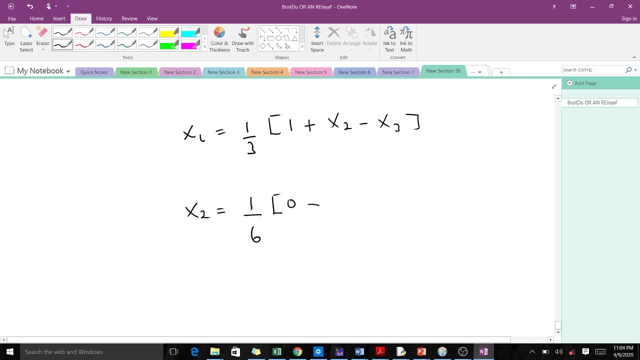 to one over six, multiplying zero minus three x one and minus two x three. then in making s3 the subject in equation three, you end up with one over seven times four minus three x one, then minus three x two. so this is the first thing we do. 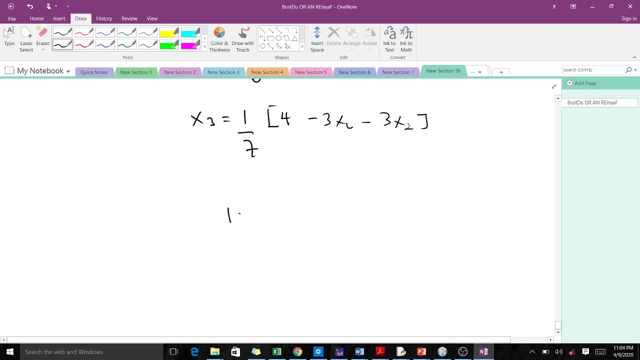 then, after that, we start with our iterations. so we are doing three iterations in this case. so with our first iteration, remember our initial condition is: s of zero equals zero, zero, zero. remember, this is our x one, x two and x three. so with the first iteration, our 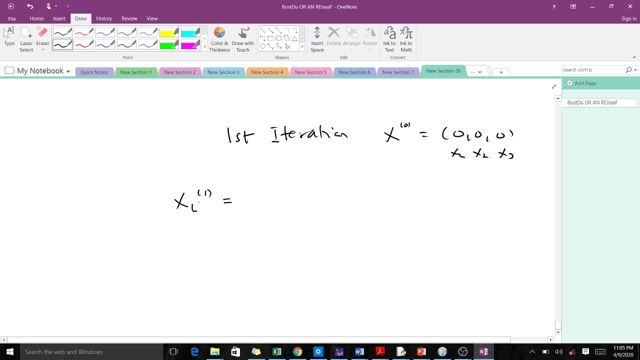 x one of one. one here, because you are doing the first iteration, will be equal to one over three, multiplying one plus x, two of zero, minus x three of zero. wondering how we got this equation. remember we made s1 as service in equation one and the new thing here is the one you can see here: the zero. 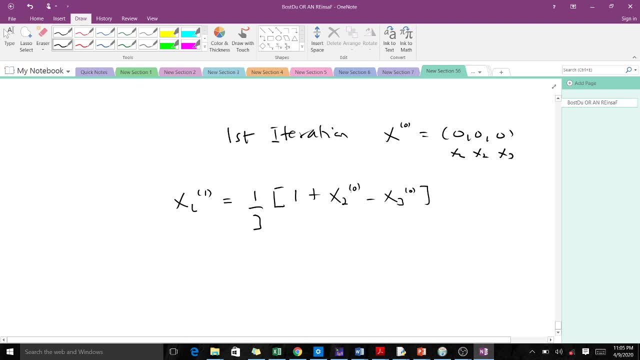 you can see in the zero. so this one means you're finding a new value for x1 using the initial condition given to us or the previous values for the x. so this is going to give you our x. one of one will be equal to one over three, one plus- remember this is zero. this is also zero. so this gives us one over three. 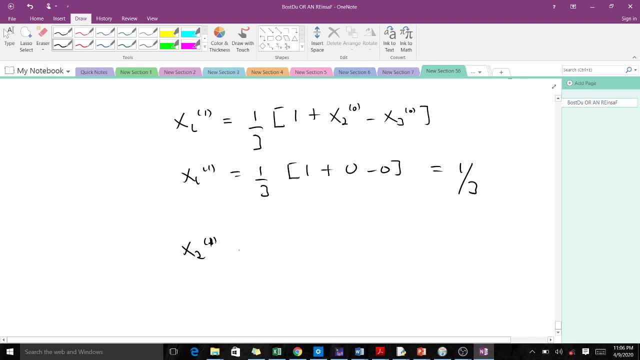 then in doing uh, finding the value for x2, so x2 we are going to get one over six. then zero minus three x one or zero minus 2 X 3 of 0, remember, everything here is 0. so when we do day, I'm going to 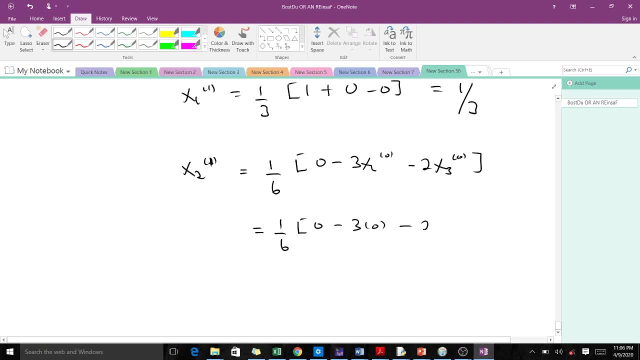 get 0 minus 3 times 0, then minus 2 times 0 and he's going to give us 0 when you go to our X 3 of 1. so we made s 3, the subject in equation 3, don't forget so. 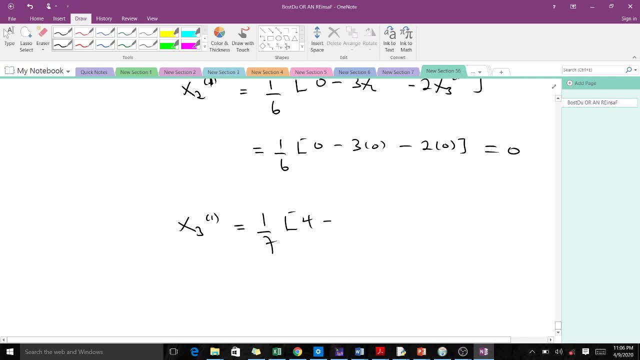 they're going to get 1 over 7, then 4 minus 3 X 1 of 0, then minus 3 X 2 of 0. so remember this piece, preserve this piece of the zeros. you are going to end up with 4 over 7. so you realize that after doing the first iteration, our new 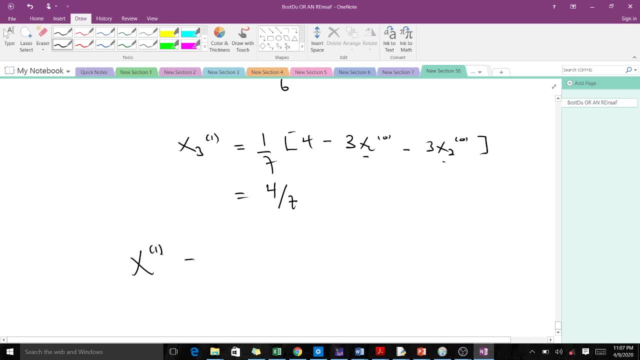 set of values for our X, that's X 1 is 1 over 7, sorry, 1 over 7, 3. so is 1 over 3, 0 and 4 over 7. so in doing a second iteration we use the values for the first iteration to get our values in the second iteration. so 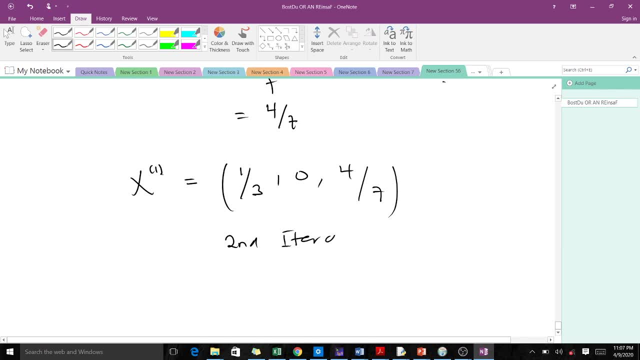 let us do the second iteration. so in doing a second iteration, we are going to get our first iteration. so in doing a second iteration, we are going to get our first iteration. so in doing a second iteration, so in doing a second iteration, we are going to get our first iteration. so in doing a second iteration, so in 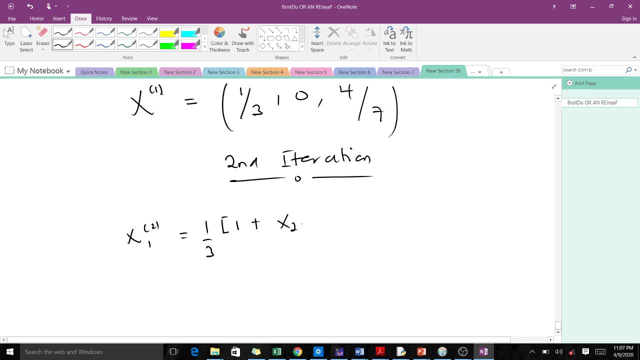 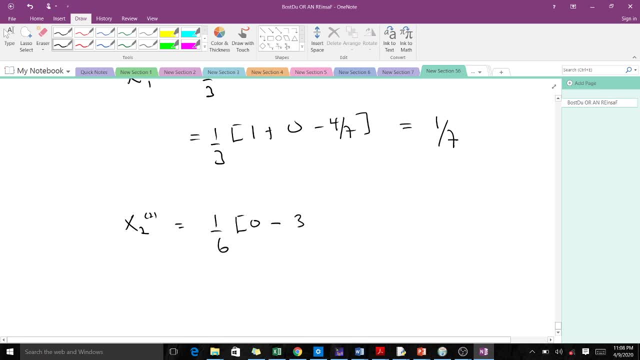 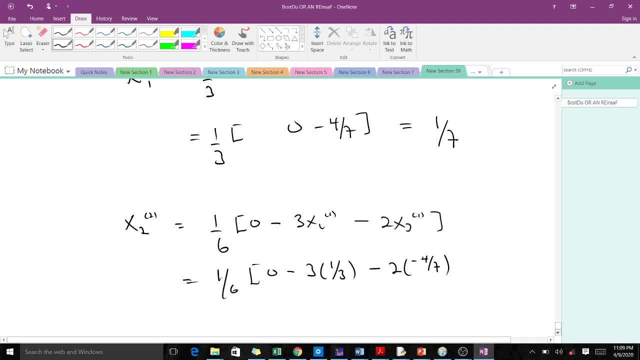 so negative 4 over 7. so remember there is, there is, there is one, here one. so when you do this computation we end up with negative 5 over 14. then find for X 3 for the second iteration. so this will be 1 over 7 and 4 minus 3. X, 1, 1 and. 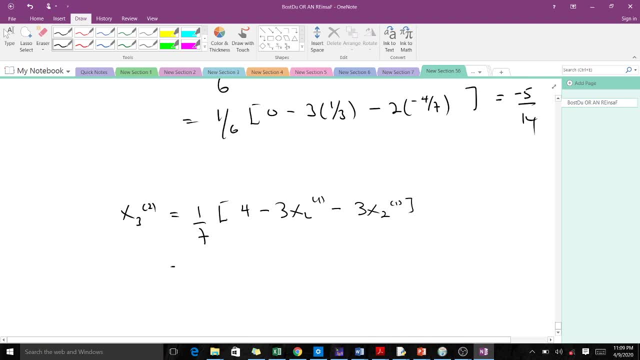 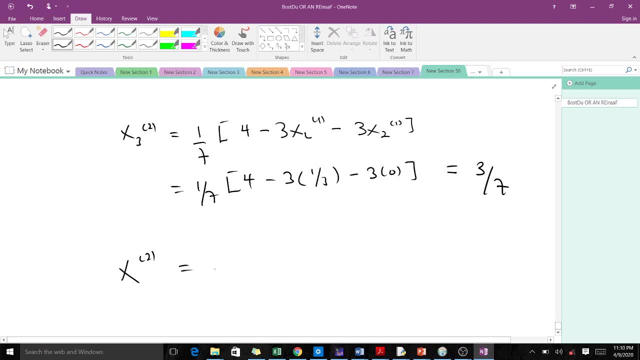 3 over 7. so that means after the second iteration. this tool: here our value for the second iteration. this tool: here our value for the second iteration. this tool: here our value for X's are 1 over 7 negative, 5 over 14. X's are 1 over 7 negative, 5 over 14. 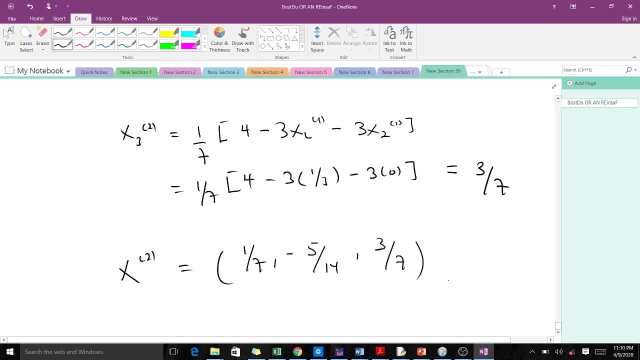 X's are 1 over 7 negative 5 over 14 and 3 over 7, then let's do the last. and 3 over 7, then let's do the last, and 3 over 7, then let's do the last iteration as a 10 iteration. so remember. 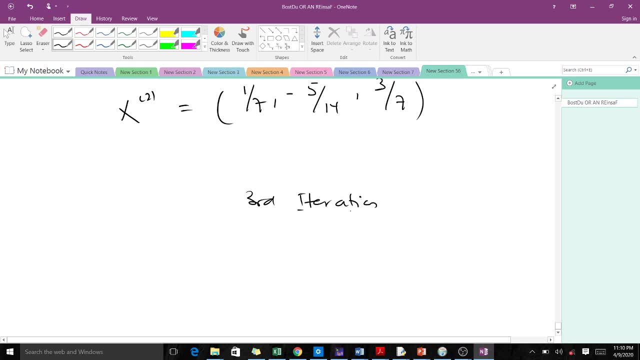 iteration as a 10 iteration, so remember iteration as a 10 iteration. so remember we use the values from the second, we use the values from the second. we use the values from the second iteration to get our values in the 10 iteration, to get our values in the 10. 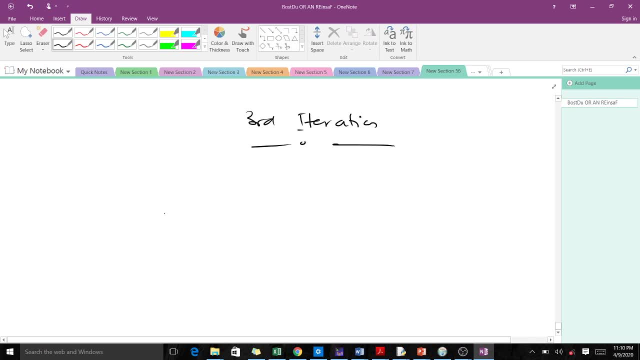 iteration to get our values in the 10 iteration. so you have our X 1 for the 10 iteration, so of 3. our X 1 for the 10 iteration, so of 3. our X 1 for the 10 iteration, so of 3, will be equal to 1 over 3 multiplying 1. 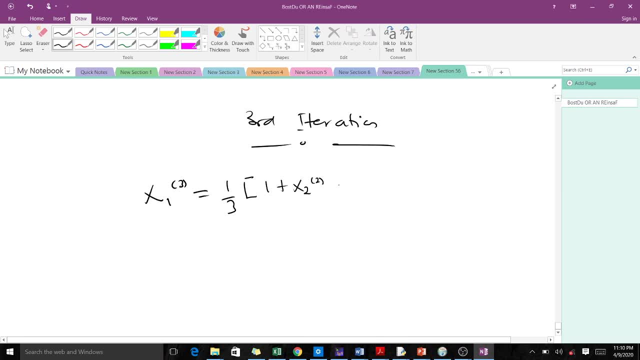 will be equal to 1 over 3 multiplying 1 will be equal to 1 over 3, multiplying 1 plus X 2 of 2 minus X 3 of 2. so this: plus X 2 of 2 minus X 3 of 2. so this: 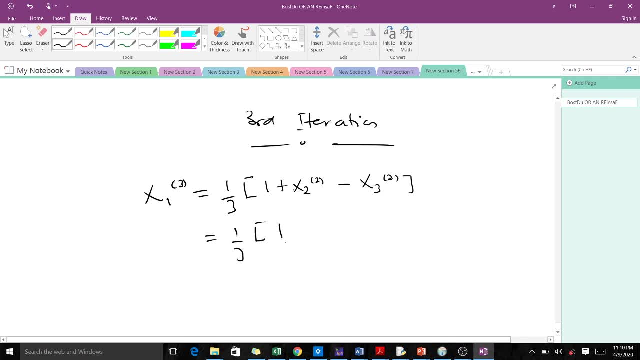 plus X 2 of 2, minus X 3 of 2, so this will give us 1 over 3: 1, but remember. will give us 1 over 3: 1, but remember. will give us 1 over 3: 1, but remember, this is minus 5 over 14. 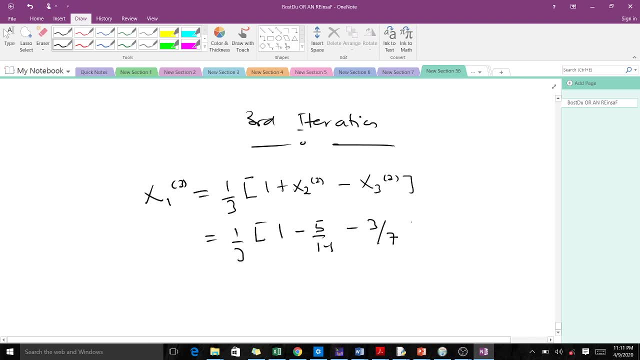 this is minus 5 over 14, this is minus 5 over 14 and this is minus 3 over 7. so when we do, and this is minus 3 over 7, so when we do, and this is minus 3 over 7, so when we do this computation and operate 1 over 14, 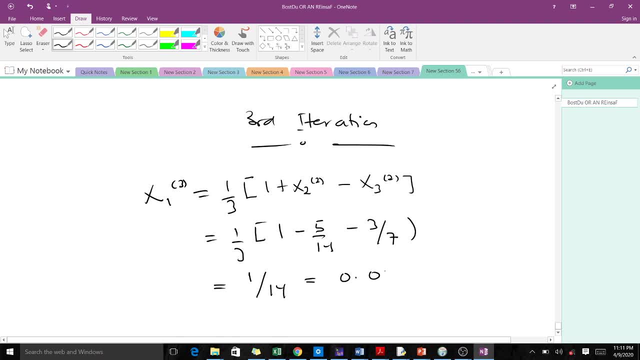 this computation and operate 1 over 14. this computation and operate 1 over 14, which is equal to 0 point, 0, 7, 1, 4. when, which is equal to 0 point 0, 7, 1, 4. when, which is equal to 0 point 0, 7, 1, 4. when you find 4 X, 2, you're going to get 1. 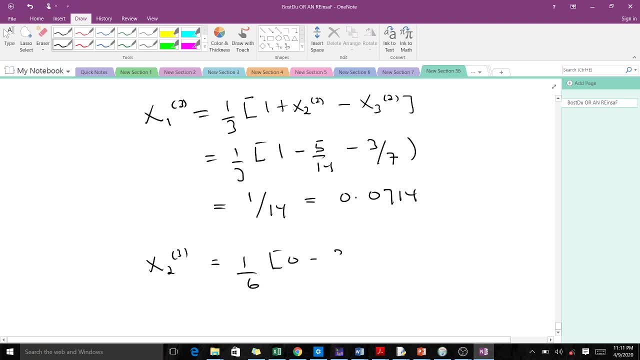 you find 4 X 2, you're going to get 1. you find 4 X 2, you're going to get 1 over 6: 0 minus 3 X 2 of 1, then minus 2. over 6: 0 minus 3 X 2 of 1, then minus 2. 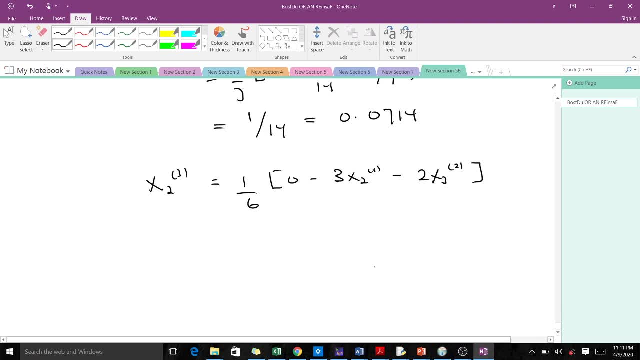 over 6: 0 minus 3, X 2 of 1, then minus 2 X 3 of 2, and when you put in the values X 3 of 2 and when you put in the values X 3 of 2, and when you put in the values for X 2 of 1 and X 3 of 1, we end up. 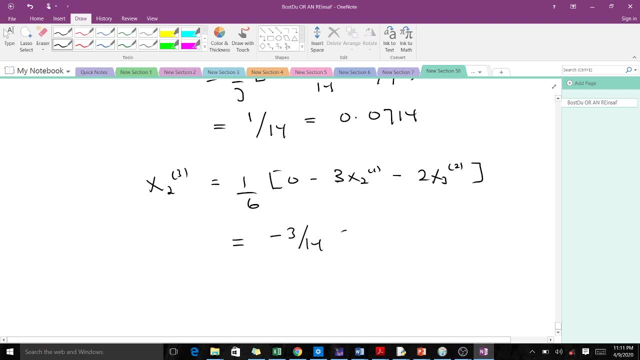 for X 2 of 1 and X 3 of 1. we end up for X 2 of 1 and X 3 of 1. we end up with negative 3 over 14, which, in terms of: with negative 3 over 14, which, in terms of. 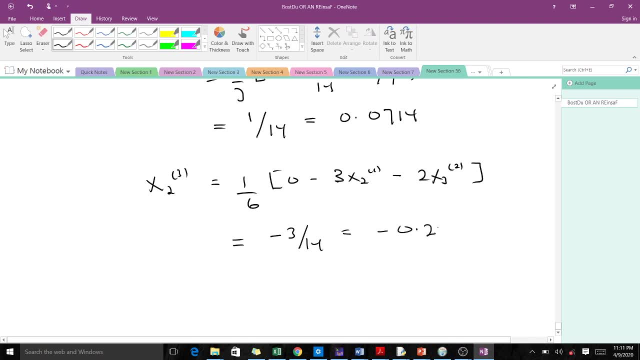 with negative 3 over 14, which in terms of decimal is negative 0. point 2, 1, 4, 3. then decimal is negative: 0. point 2, 1, 4, 3. then decimal is negative: 0. point 2, 1, 4, 3. then to get our X 3 for a tail iteration, we 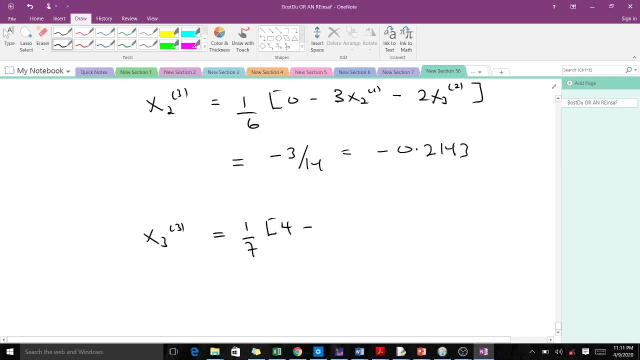 to get our X 3 for a tail iteration. we to get our X 3 for a tail iteration. we get 1 over 7 and 4 minus. get 1 over 7 and 4 minus. get 1 over 7 and 4 minus. so this will be 3 X 1 for the second. 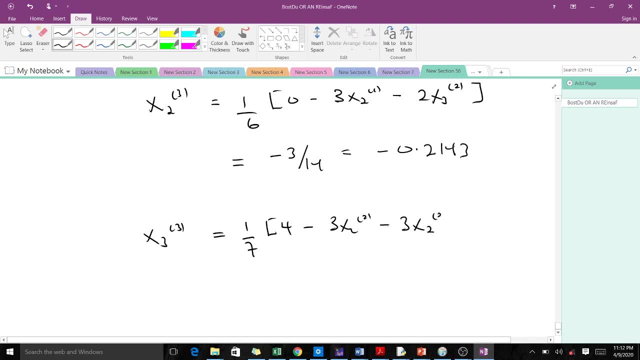 so this will be 3 X 1 for the second. so this will be 3 X 1 for the second iteration and 3 X 2 for the second iteration, and 3 X 2 for the second iteration and 3 X 2 for the second iteration as well. and this gives us when. 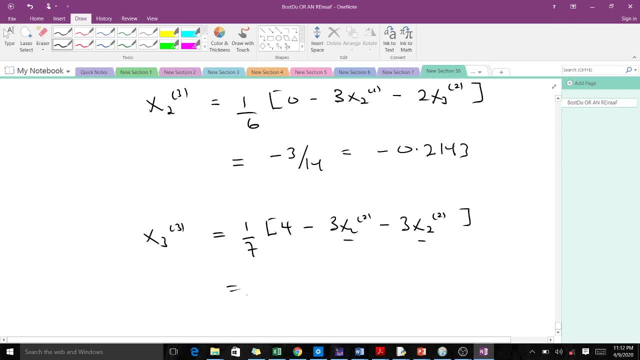 iteration as well, and this gives us when iteration as well, and this gives us: when you put in the value for X 1 and X 2, for you put in the value for X 1 and X 2, for you put in the value for X 1 and X 2 for the second iteration, this one gives us. 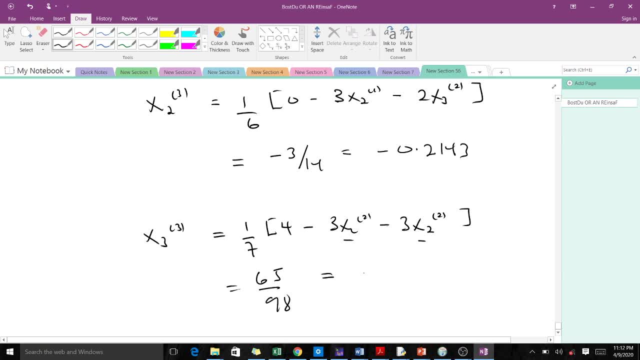 the second iteration. this one gives us the second iteration. this one gives us 65 over 98, which is equal to 0.6633, so 65 over 98, which is equal to 0.6633, so 65 over 98, which is equal to 0.6633. so since 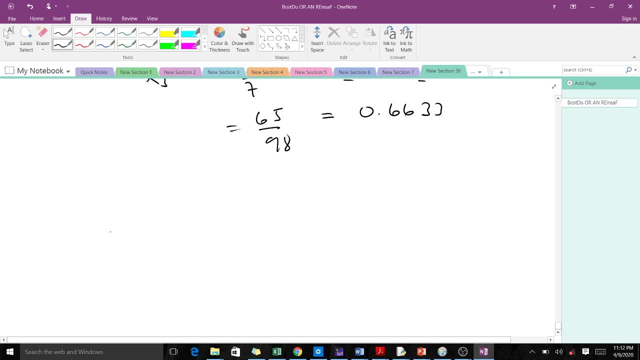 since, since. since the question asks us to do only 3, the question asks us to do only 3. the question asks us to do only 3. iteration that means our pros meted. iteration, that means our pros meted. iteration, that means our pros meted. remember, we did I tuition, so when we get 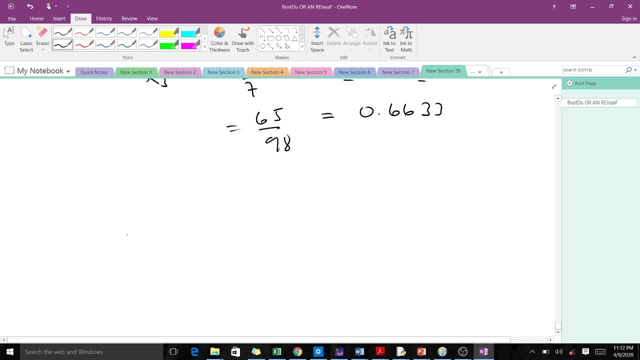 remember we did I tuition, so when we get, remember we did I tuition, so when we get, the outside is not pros meted solution. the outside is not pros meted solution. the outside is not pros meted solution. so our pros meted solution to the system. 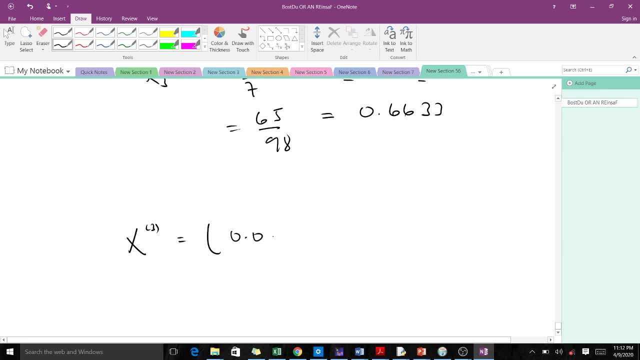 so our pros meted solution to the system. so our pros meted solution to the system of linear equation. there is 0.0, 7, 1, 4 of linear equation. there is 0.0, 7, 1, 4 of linear equation. there is 0.0, 7, 1, 4 comma, negative, 0, point, 2, 1, 4, 3. then 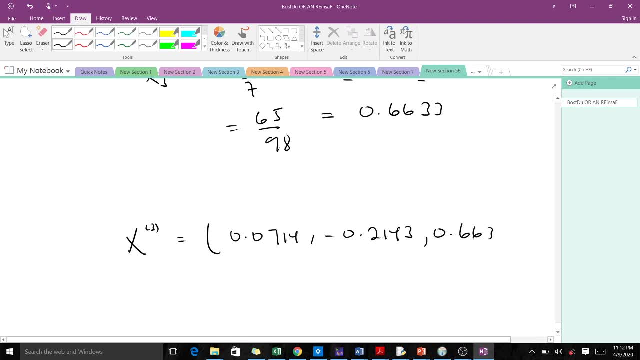